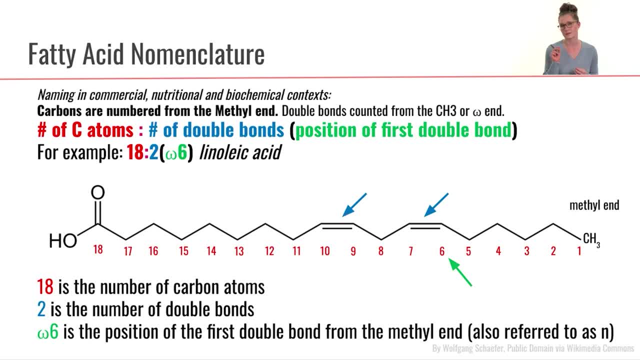 the most important context for us, and then I'll talk about how they name things a little bit differently in the chemistry world. So first of all, when we are naming a fatty acid, we want to know how many carbons are in it. So we want to count the number of carbons. The next thing we 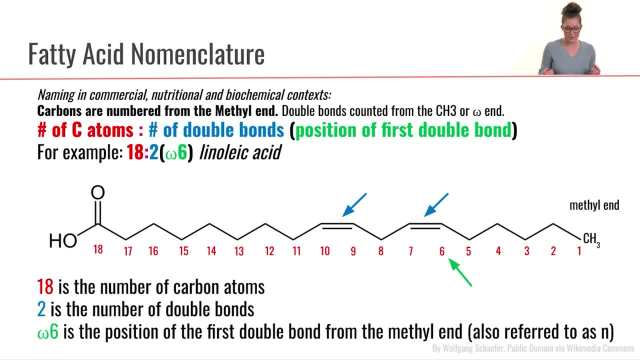 want to know are how many double bonds there are, because that, we know, is going to be very important for the function of our fatty acid. And then, third, we want to know where is the first double bond. Now, in order to know where the first double bond is, we need to count our fatty acids in our tail. 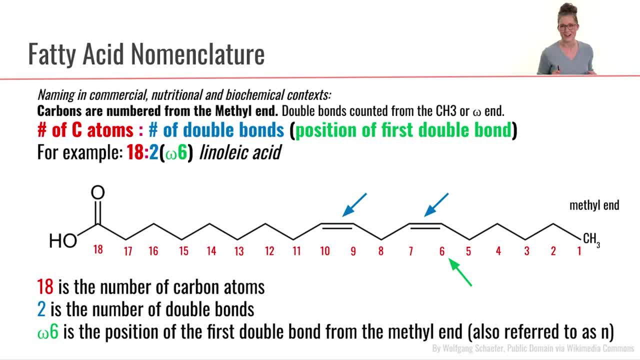 So when we are count or we need to count the carbons- pardon me, in our fatty acid tail. So when we are counting the carbons in our fatty acid, we have to know which end to start at. Which end counts as number one When we are in this. 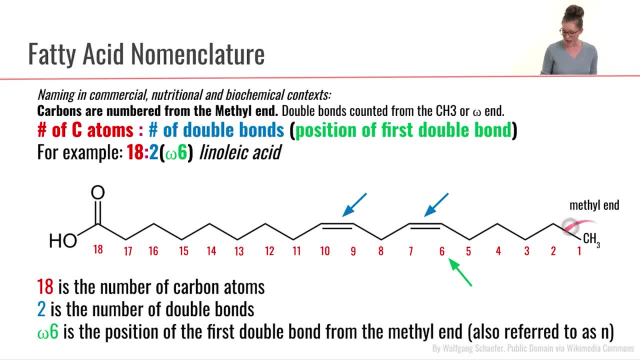 commercial, nutritional, biochemical area. we count the methyl end of our fatty acid tail as carbon number one. So in this example here we would start to name this particular fatty acid, we would start by counting at the methyl end. So that's one. we see that we end up with one, two, three, four, five. 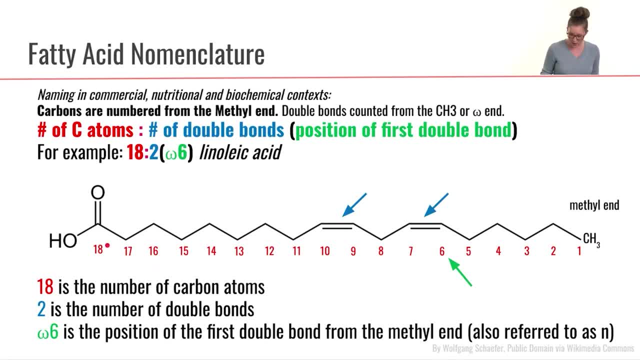 six, seven, all the way up to eighteen carbons total. We see that we have two double bonds Here. Then we see that our first double bond comes at carbon number six. Now the other specific nomenclature that is used here is the term: 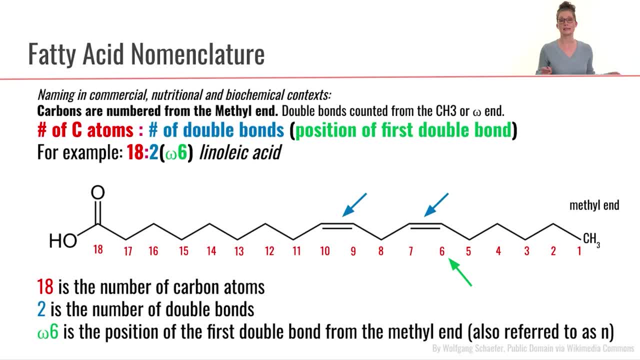 omega. Now think back to the greek alphabet. omega is the last letter in the greek alphabet, So we use the term omega to say how far away we are from from the end. So in this case, this would be that we would use the term omega to denote where the 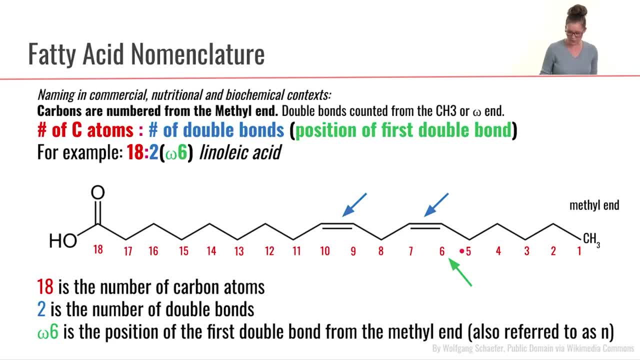 first double bond is: And so in this case our first double bond is at carbon number six, So we would call this an omega-6 fatty acid. So putting all of that together, this fatty acid here would be named as 18-2-omega-6.. And that turns out that this happens to be linoleic acid, one of our 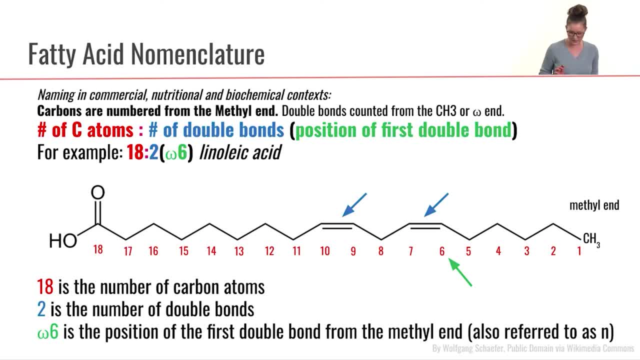 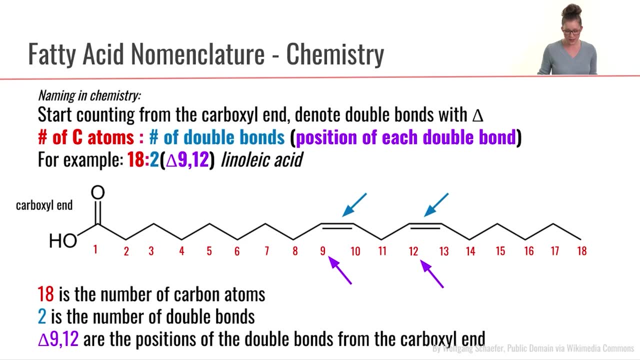 essential fatty acids. So that is how we name things in kind of mostly in the nutrition text. Now, frequently you will also notice that omega is sometimes abbreviated as N, So we would just say our N6 fatty acids. So that's something to keep aware of in the literature. Now, as I mentioned,